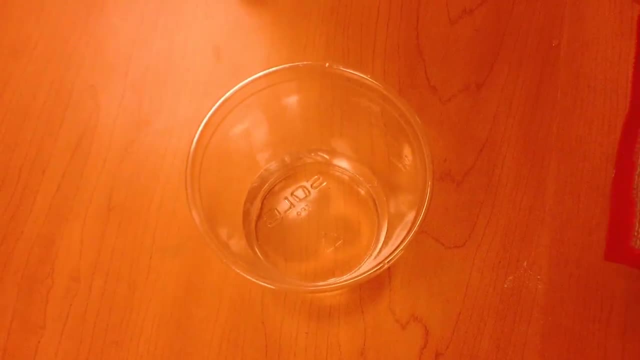 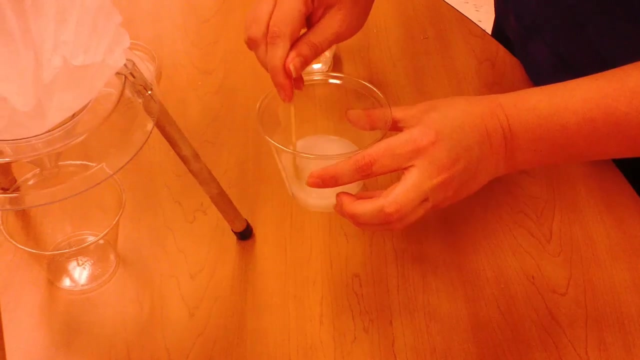 you have the gravel and there's the water. It's been separated. Sometimes you have a mixture where the particles are smaller. This is a mixture of water and powder. The screen has holes that are two or three inches in diameter. If you have a mixture of water and powder, you can separate. 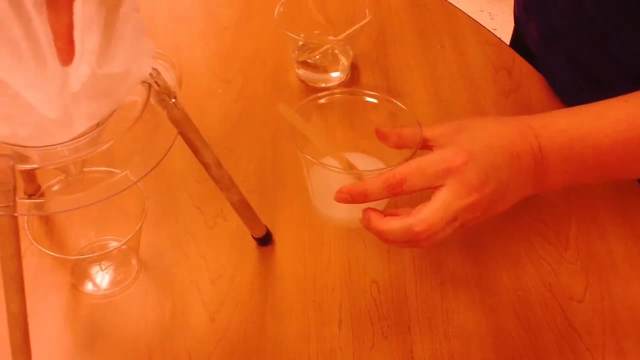 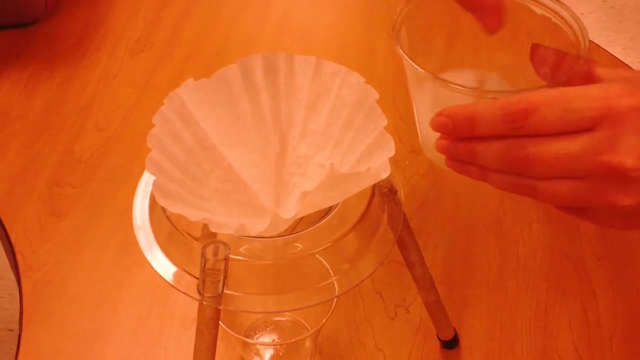 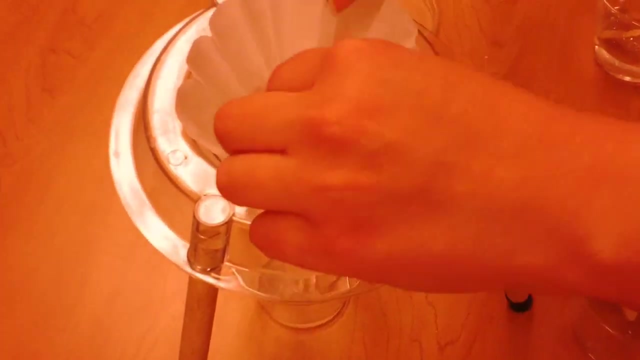 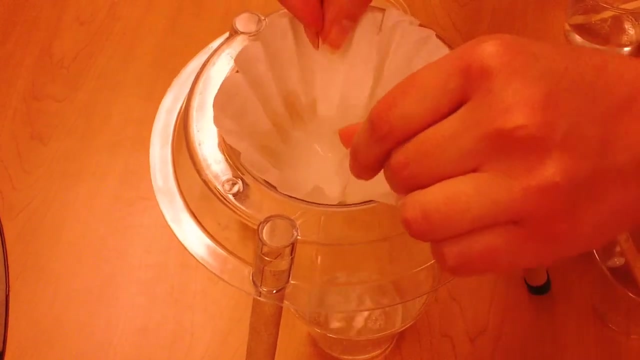 the water and powder, So we need something with smaller holes. This filter paper has smaller holes, So when I pour the water and powder mixture through, the powder gets caught in the filter paper while the clear water comes through underneath As it's getting separated, you can start to see the powder is getting clumped up and stuck. 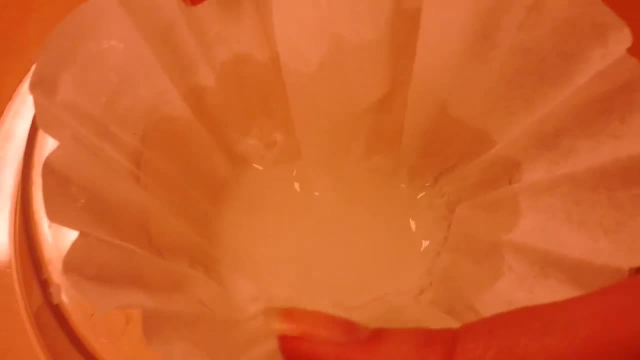 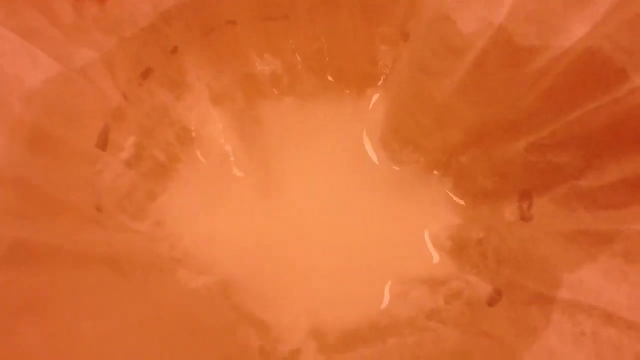 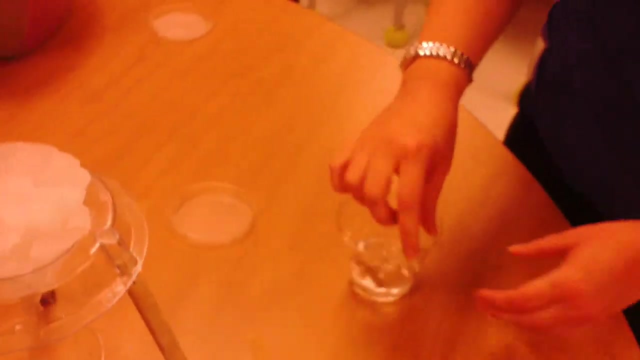 in that filter paper and the clear water is coming through the bottom. Almost all of this powder is getting separated out and stuck in the filter paper. Sometimes you have a special kind of mixture called a solution. This is a mixture of salt and water And it's special because 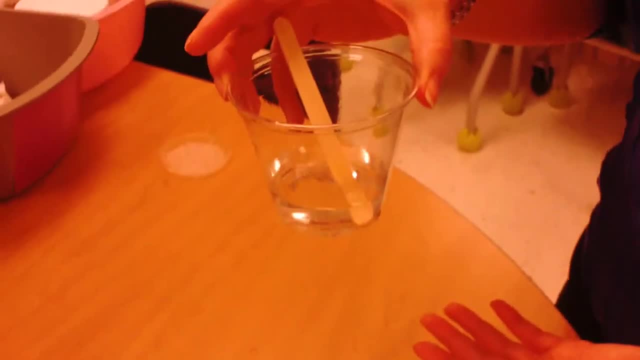 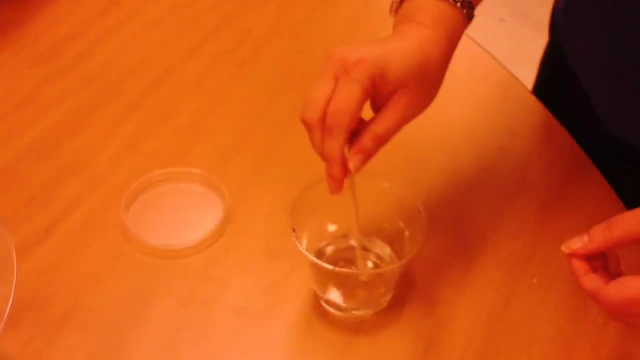 the salt dissolved in the water. We can't even see the salt anymore. This is not going to be separated by a screen or the water filter. So now you have this purple gray, appreciated solution. This is a or a filter. we need to do something different. 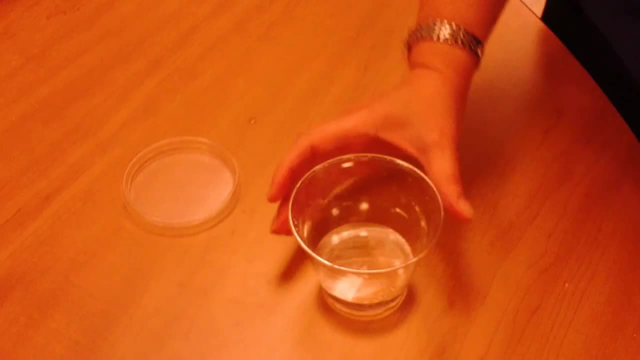 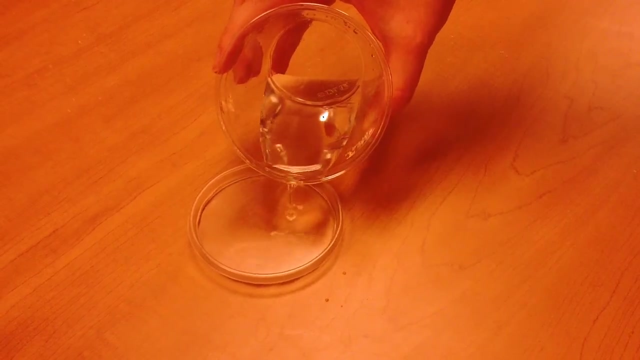 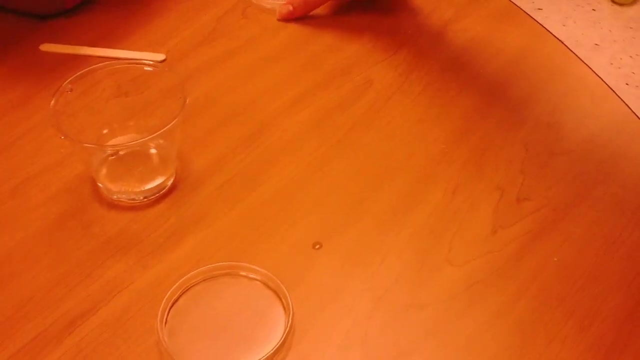 We need to set it up to evaporate. If we pour this solution into an evaporation dish and let it sit to evaporate, eventually the water will all evaporate into the air and it will leave the salt particles behind. This is what it will look like. 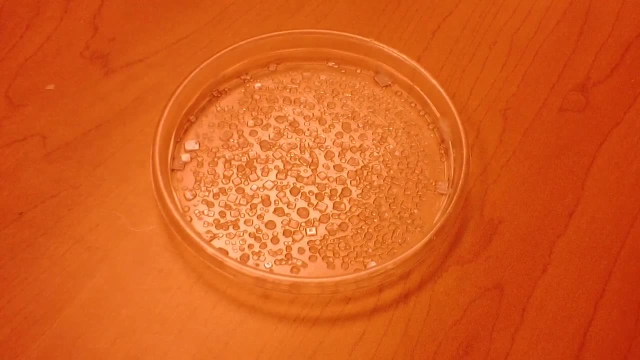 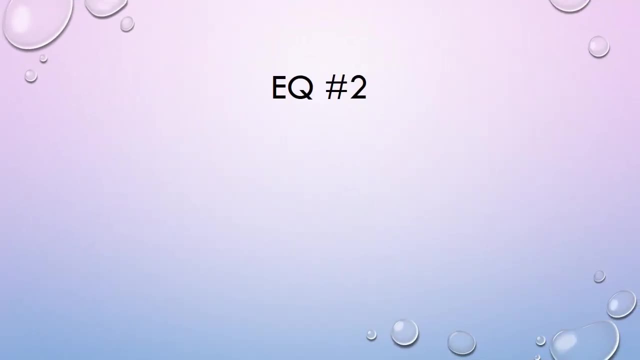 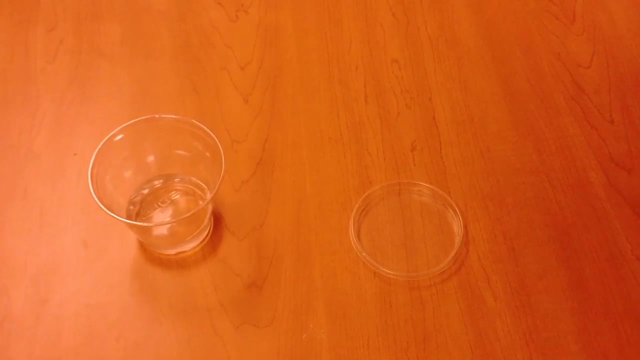 after the water has all evaporated away, It leaves the salt behind. That is how you can separate a solution. The second essential question is: how can you determine if a clear liquid is a solution? In order to determine whether a clear liquid is a solution, 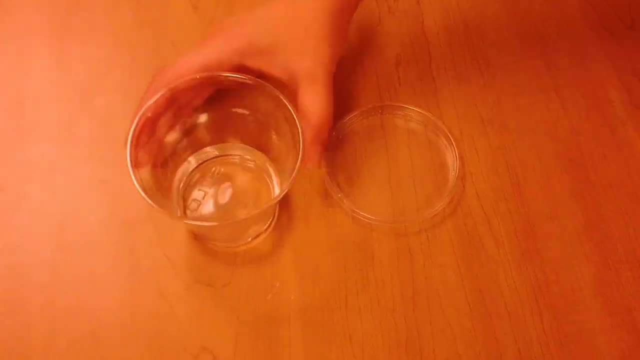 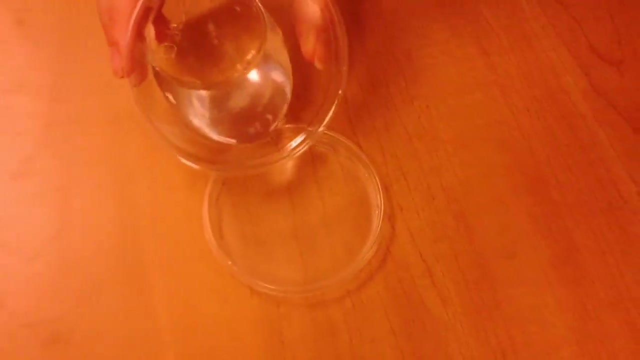 one thing you can do is evaporate it. This is a clear liquid. I'm not sure if it is just water or if it's a solution, So I'm going to pour it into this evaporation dish After I let the evaporation dish sit for a few days.